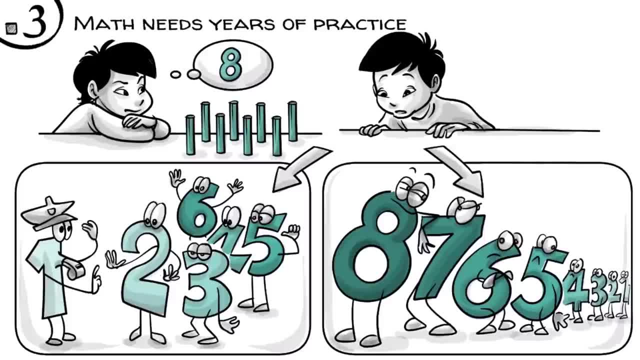 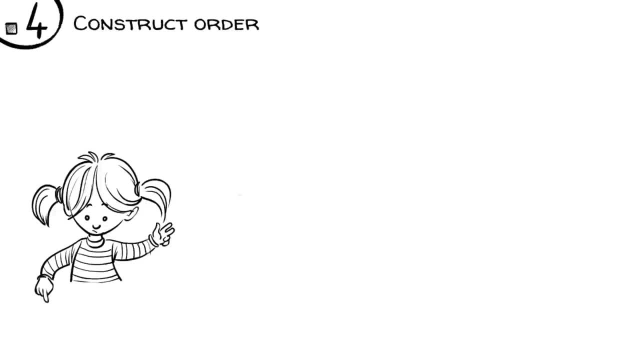 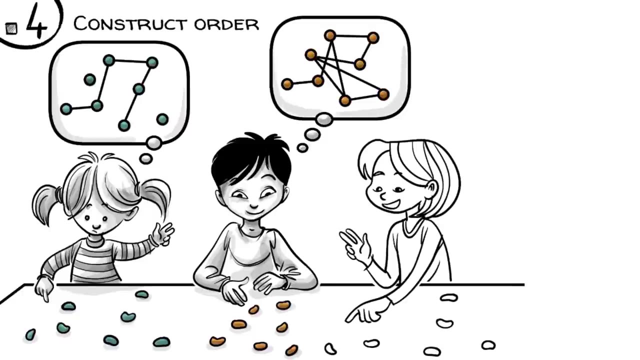 relationships. Let's look at order first: Construct order. When four-year-olds learn to count, most have trouble ordering objects in their heads if the things they count are unevenly distributed. Sometimes they skip objects. then they count the same ones twice. To do it right, children have to learn how to construct order in their heads. This seems. easy but actually takes our brains out of the box. To do it right, children have to learn how to construct order in their heads. This seems easy but actually takes our brains out of the box. So let's try to do it in a shown way. 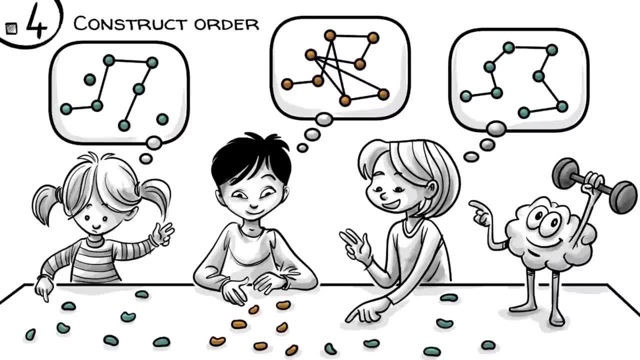 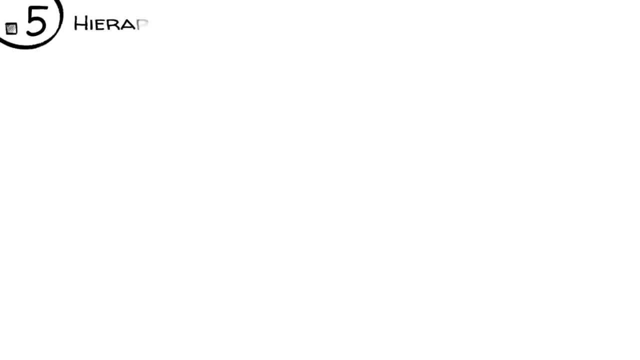 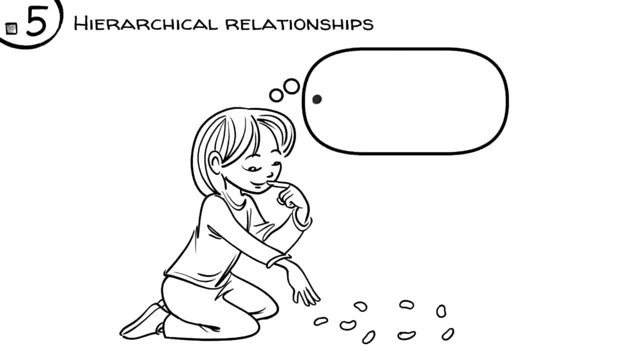 People in a lot of good health care today can say that the best set of constants comes from keeping up with the desires of everybody. Once children learn to order objects in their heads, they can put them in relationships, Hierachical relationships. As children construct, order, they count the objects as follows: 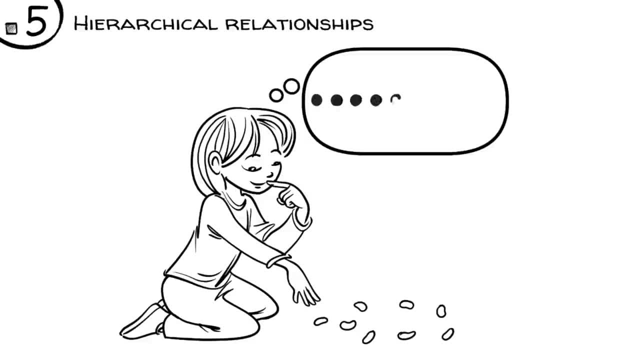 One, two, three, four, five, six, seven and eight, As they do that the number eight represents the eighth place in the order, because eight equations are creating order, As the number eight is part of its order and the objects practically the numbers of their 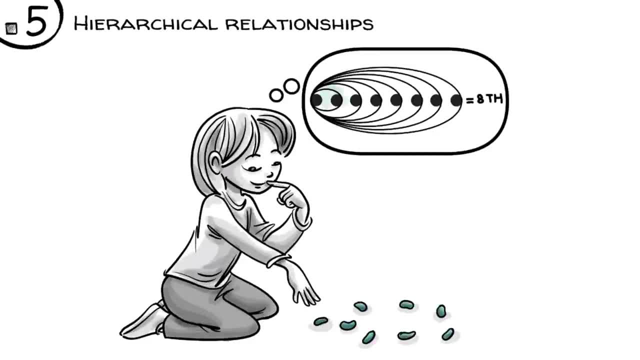 In other words, 8 always includes 1,, 2,, 3,, 4,, 5,, 6,, 7.. The idea of 8 is therefore a hierarchical relationship between the 8th object and all those preceding it. 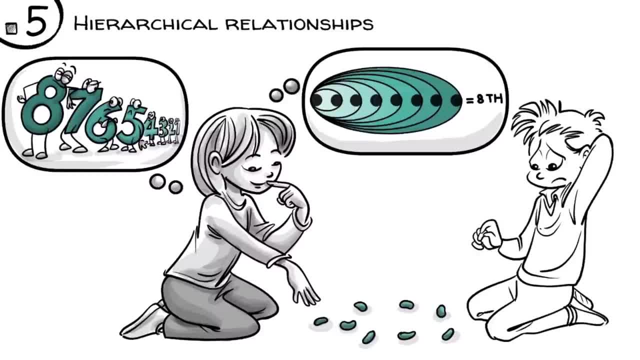 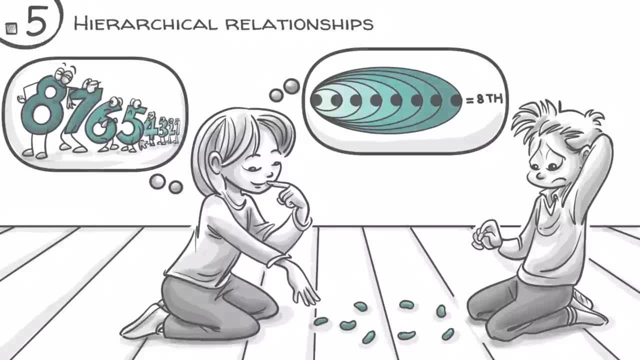 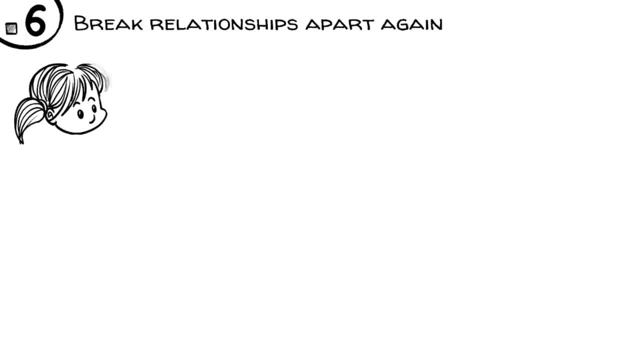 If we don't learn to do this sort of abstraction by doing lots of math in our heads, we won't be able to form a solid foundation for arithmetic. After building them, children need to learn to break relationships apart again. We can see how hard this is when we present a 5-year-old an image of 6 dogs and 2 cats. 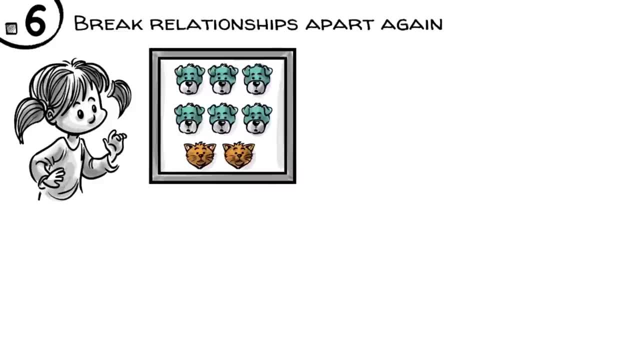 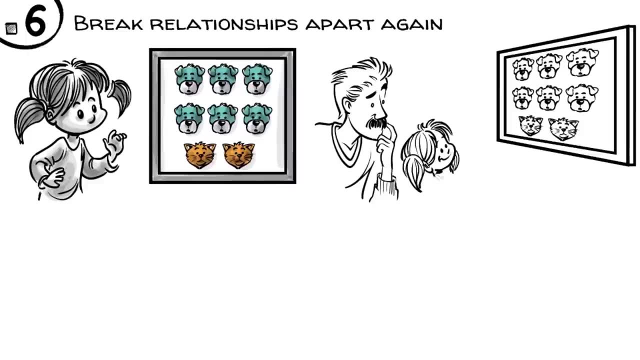 and then ask: are there more dogs or more animals? While most adults, who see the full picture, find this question odd, a 5-year-old typically just answers more dogs. When you ask further more dogs than what, The child replies then cats. 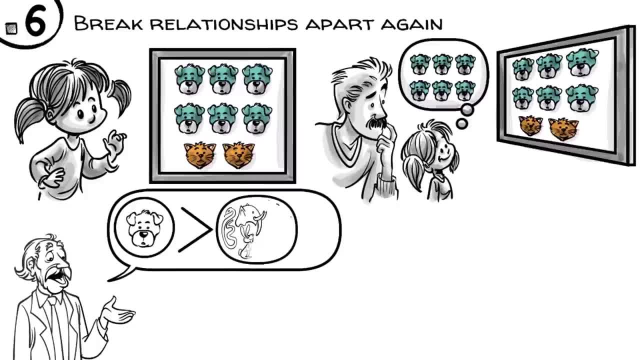 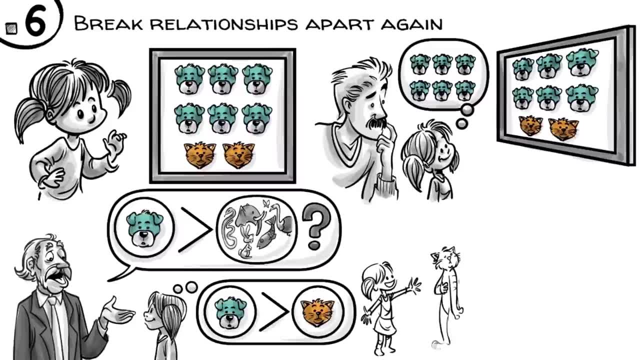 In other words, if you ask are there more dogs or more animals, The child hears: are there more dogs or more cats? At age 5, most kids didn't practice enough math to break hierarchical relationships apart while still remembering the whole. 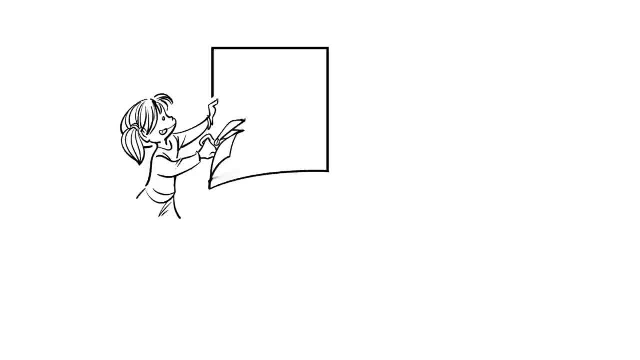 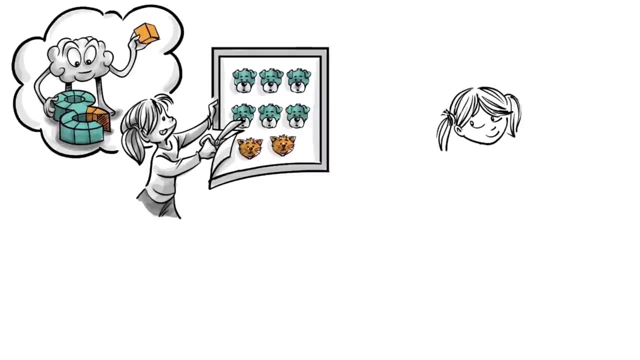 This happens because once the child has to cut the whole into parts, for them, at that moment the whole no longer exists. They have not yet constructed the concept of 8 without thinking of it as a sum of its parts. So when they divide the animals into cats and dogs, 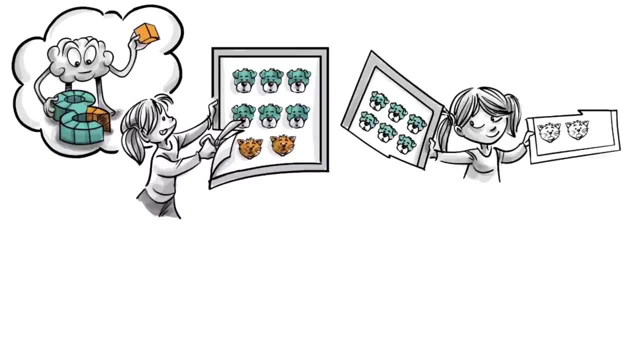 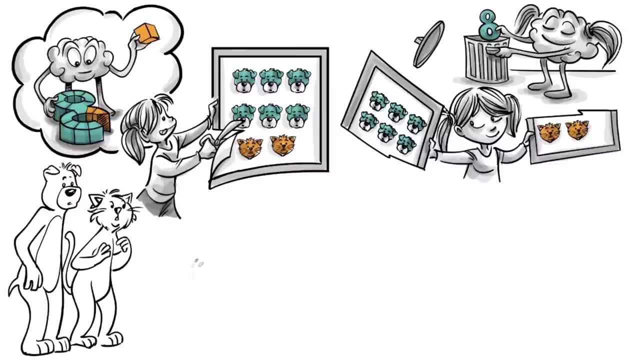 all they can think of are two parts, of which one looks larger. The idea of 8 is then forgotten. To also think about all animals would require two opposite mental actions: First, divide the whole and then put it back together, a mental process that most 5-year-old children precisely can't do. 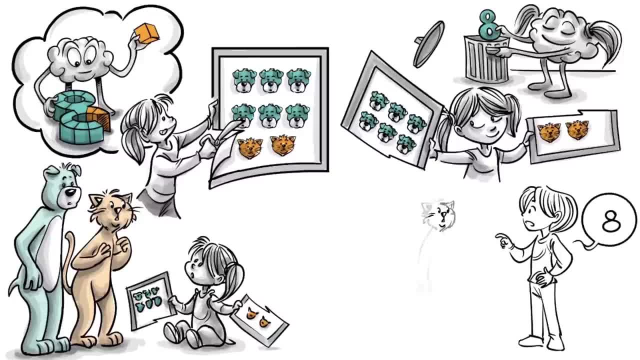 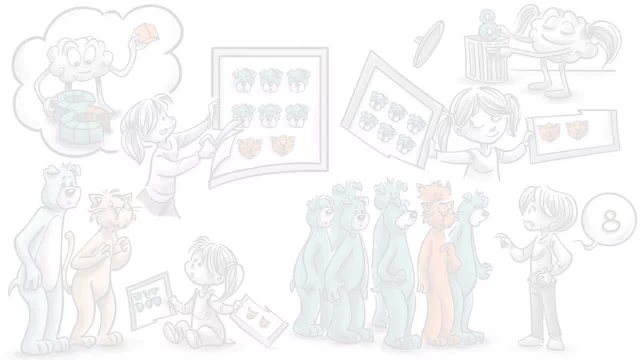 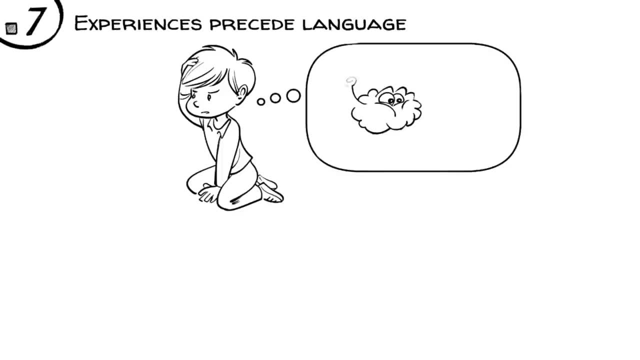 Only by age 7, most children can see the whole and keep its abstraction in their heads and still divide the sum in its parts. As we demonstrated, it takes a child a lot of mental training and hands-on experiences to form the concept of a number. 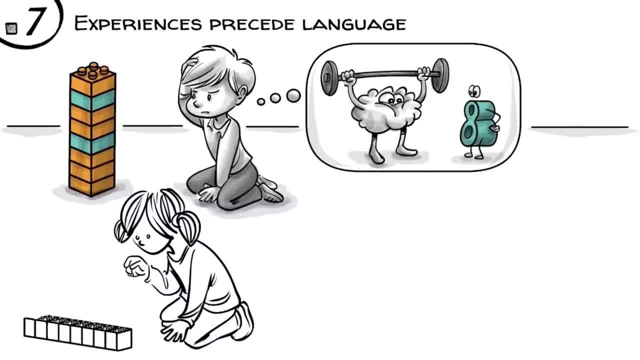 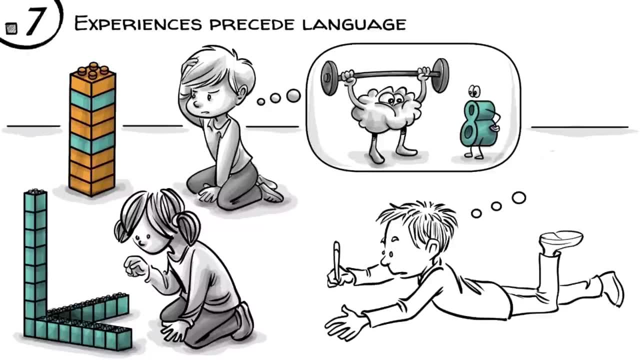 At the age of 5, the child can only see the whole of five. we can build a simple row of eight, later form eight square, then eight root. only once we have constructed number concepts inside our heads can we effectively learn how to express them with. 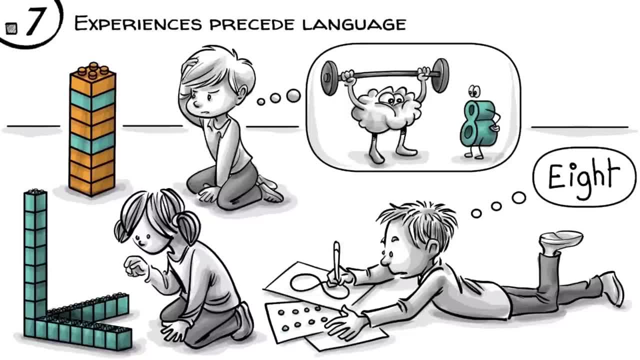 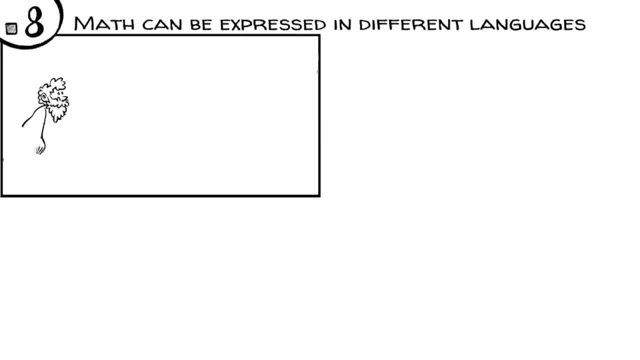 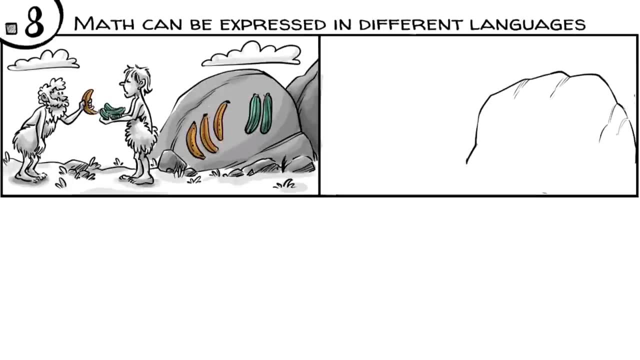 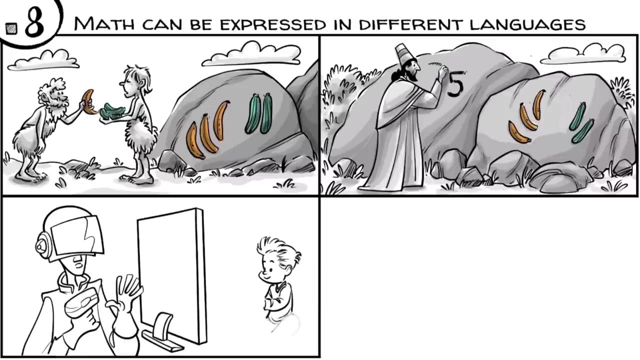 images, symbols and language. math can be expressed in different languages. a hundred thousand years ago, we used objects to express our mathematical thinking. later we used images. around 1 000 years ago, we began to reduce images to arabic numeral symbols. in future, we might replace symbols with: 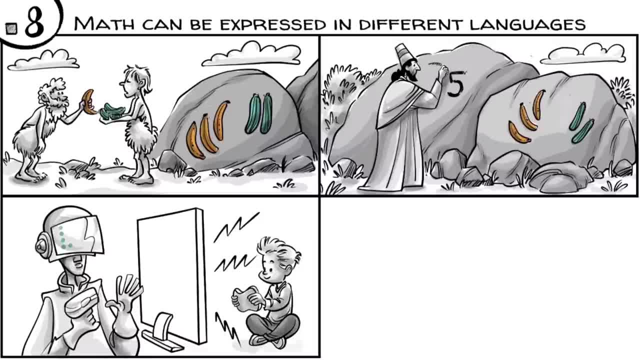 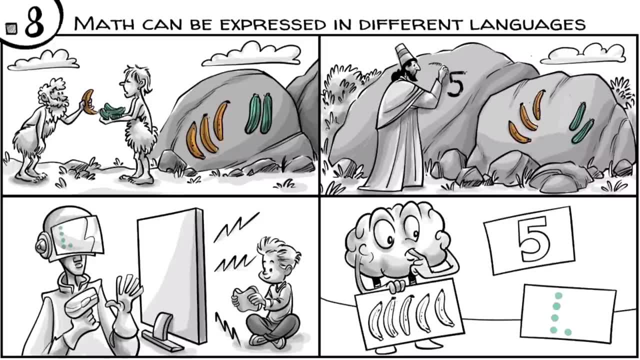 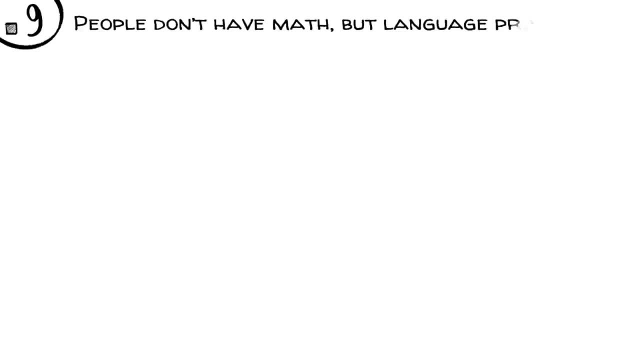 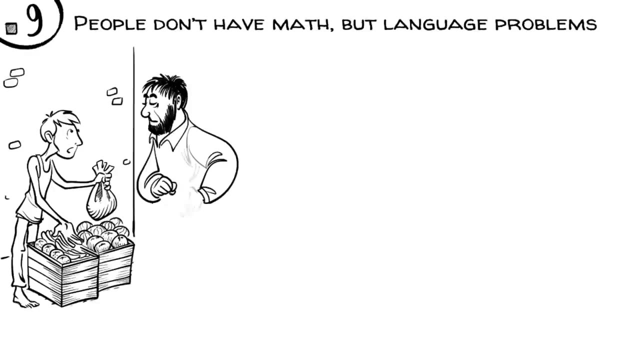 bits or express math in graphic simulations or games. in other words, while math thinking always happens in our heads, the language that represents our thinking is evolving. most people don't have math but language problems. we know, for example, that 11 year old unschooled street vendors are often highly proficient in complex money transactions, but incapable of doing. 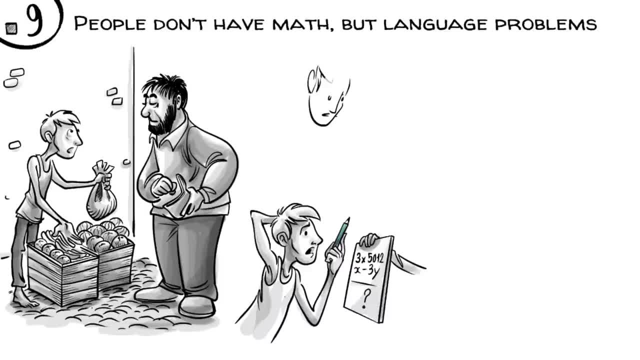 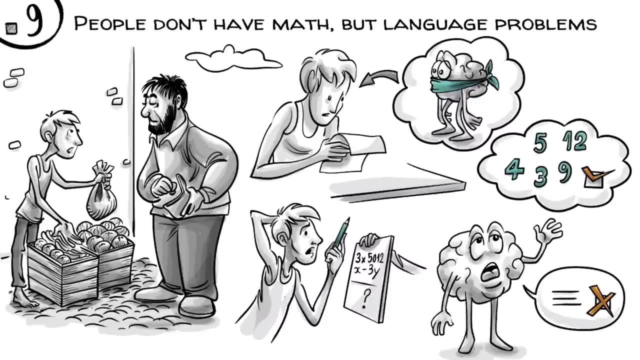 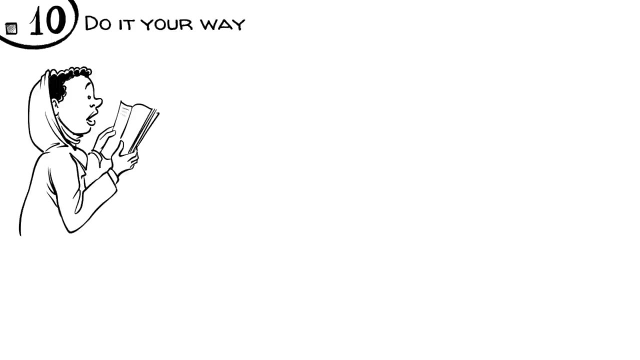 paper and pencil arithmetic. this phenomenon, known as street mathematics, shows that when smart kids struggle in school, they often just can't express their thinking in symbols. their brains can do math, but have language problems. one way to solve this is to do it your way, just like nobody ever learned to speak a language, just 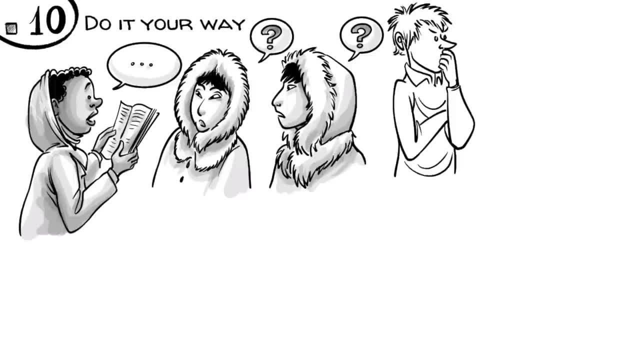 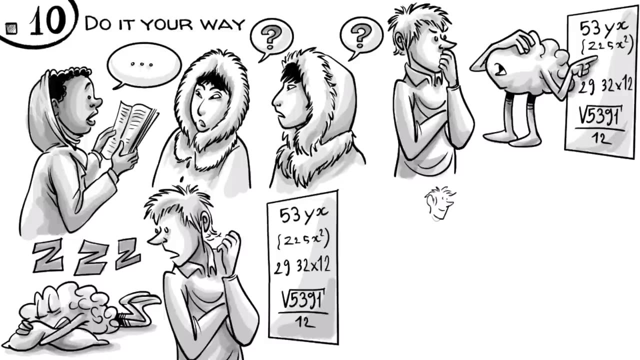 by learning the rules of grammar. nobody learns math by memorizing the rules of how to arrange numbers and symbols in order to find the right answer to a problem. whenever we do that, we stop constructing fundamental principles inside our heads. to get better and confident, children should be encouraged to find their own path and use their own language to express a 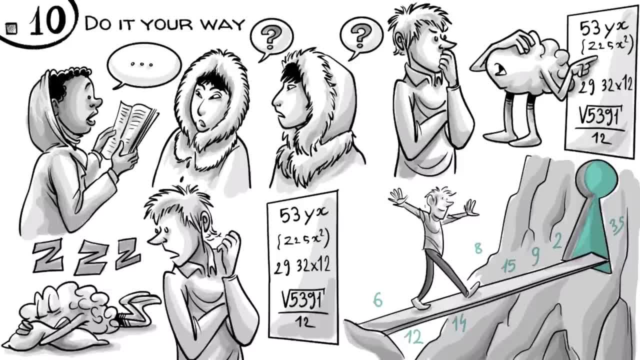 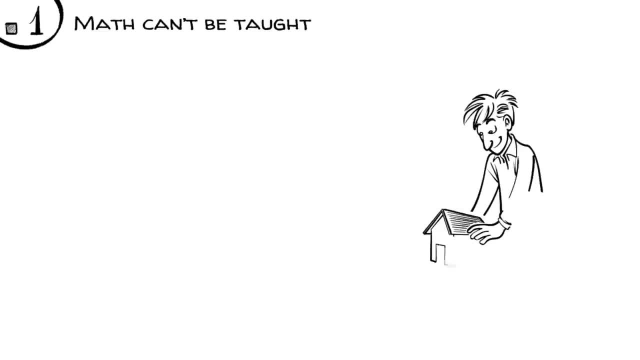 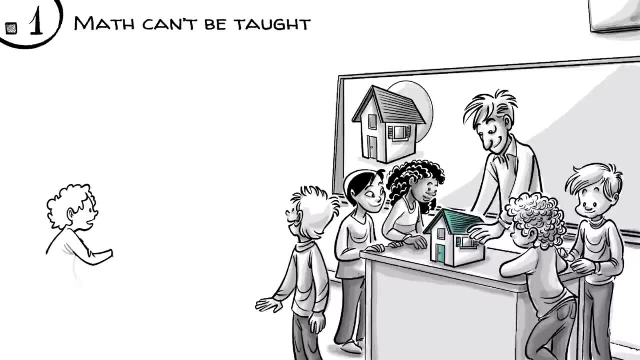 solution which brings us back to rule one: math can't be taught, it has to be constructed. if we want to learn math, we have to do math in our heads, ideally with real-life experiences. later we replace the objects with abstractions, such as language symbols or whatever. the few. 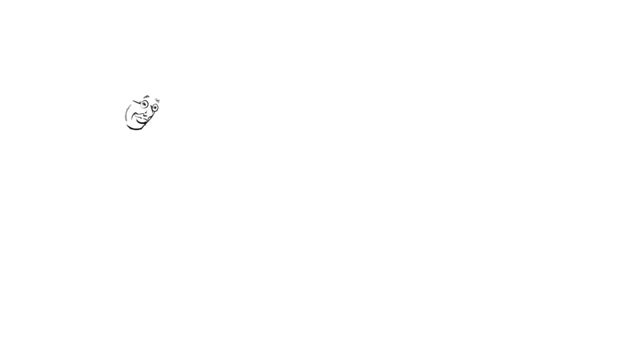 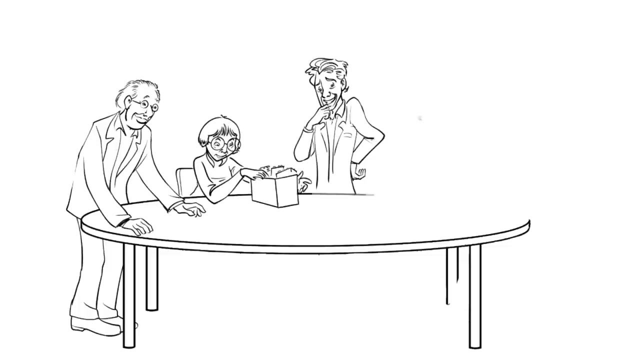 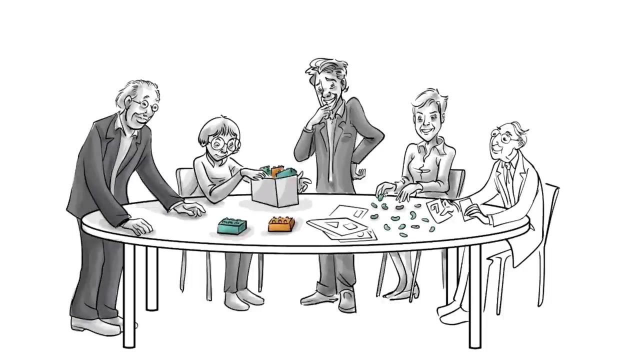 might bring. The ideas presented in this video are based on the work of Jean Piaget, Constance Camus, Keith Devlin, Georgia de Clark and Jerome Brunner, who all contributed immensely to the body of work and research on how children and 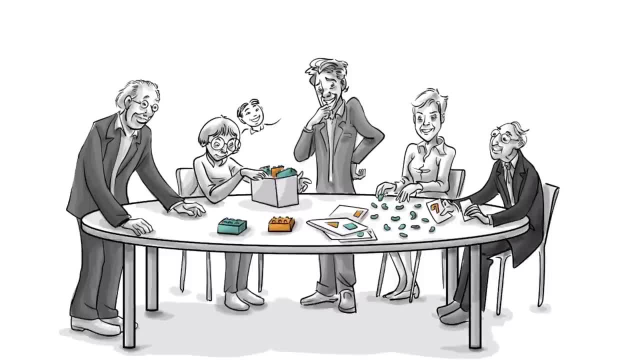 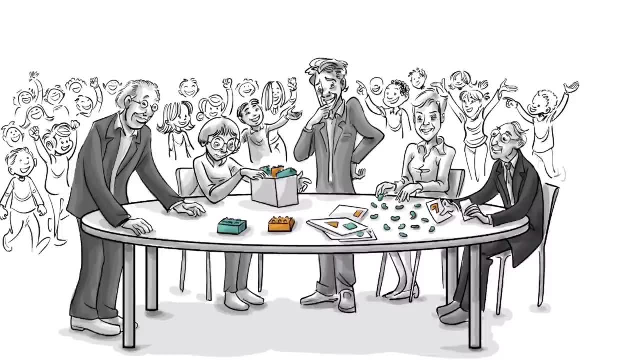 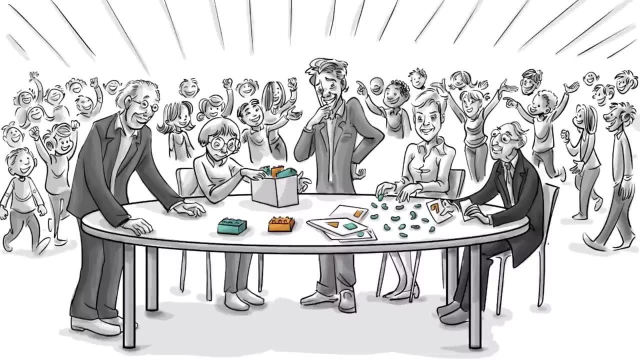 adults learn math. If you want to get better at math today, join Keith Devlin from Stanford University and over a hundred thousand students from all around the world in his free course on Thinking Mathematically. See the descriptions below for more details and links for the research. 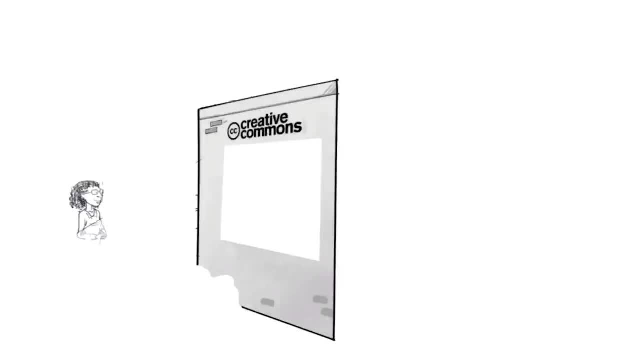 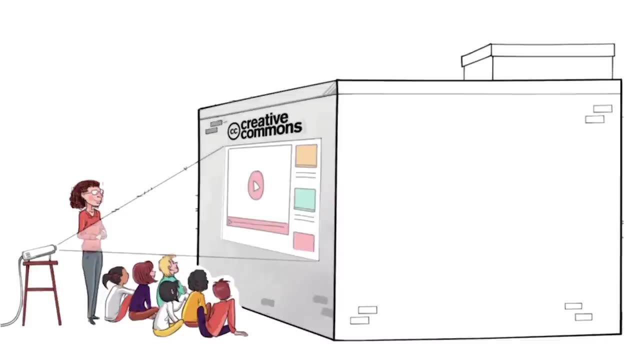 Sprouts videos are published under the Creative Commons license. That means our videos are free and any of your videos are free to watch. Anyone can download, edit and play them for personal use, And public schools, governments and nonprofit organizations can also use them for training online. 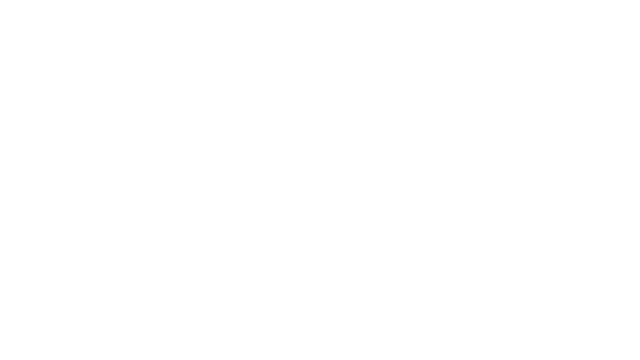 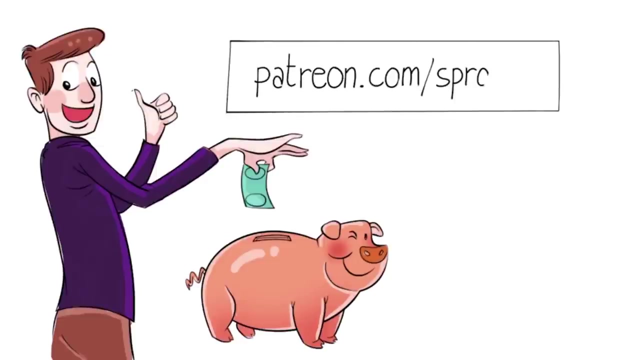 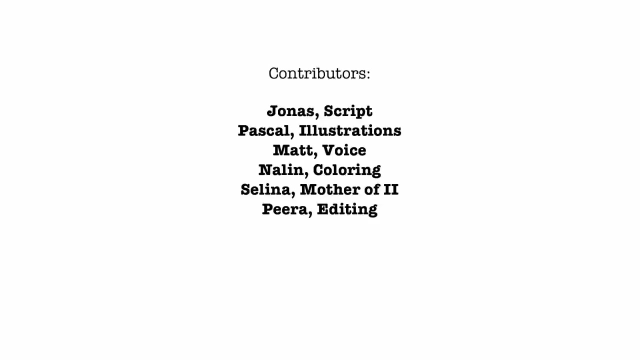 courses or designing new curriculums To help us stay independent and support our work. you can join our patrons and contribute. Just visit patreoncom slash sprouts. Even one dollar can make a difference you.